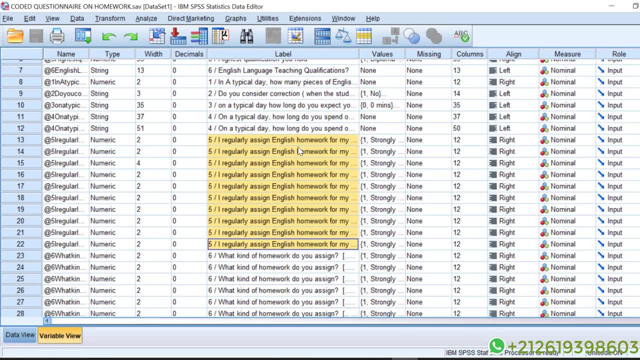 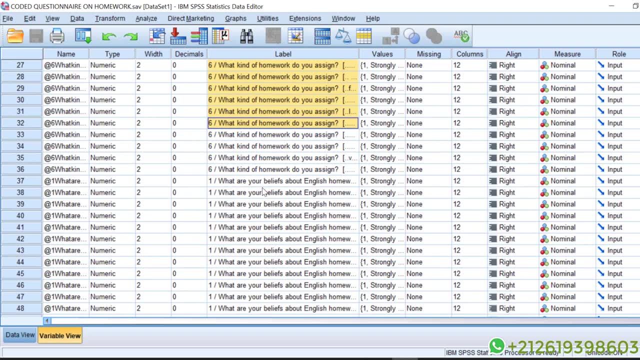 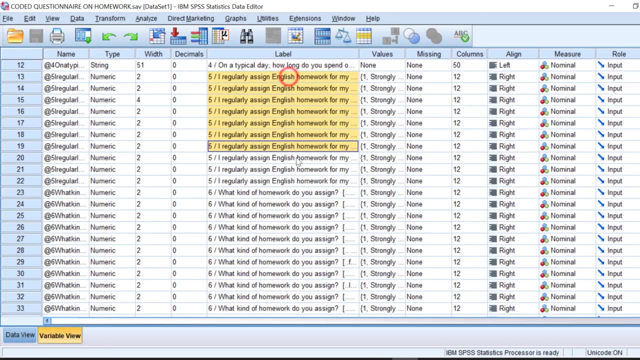 different items that correspond to a certain theme, like this regular assignment of English homework, then the kind of the assigned homework, as well as the beliefs about English homework. so what I need to do is that I need to reduce the these items of the record scale, or the seven point, or 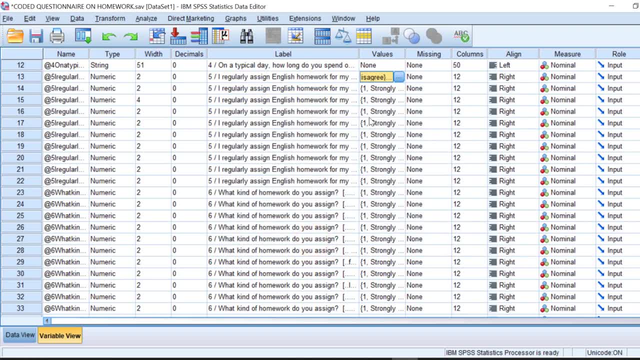 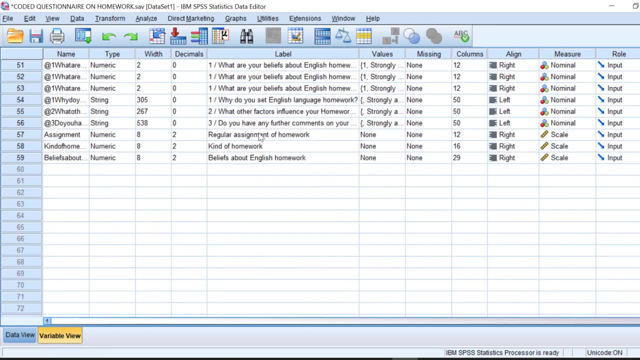 five point record scale into one variable or one group or one category like this. so I need all these items to be one like in this one, so that I can call it, for instance, regular assignment homework, kind of homework and beliefs about English homework. so there are two ways in which I can group these. 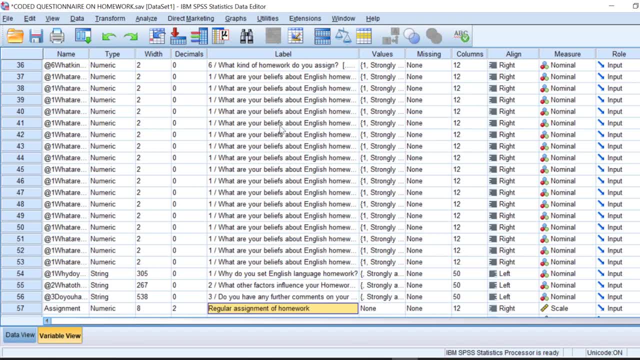 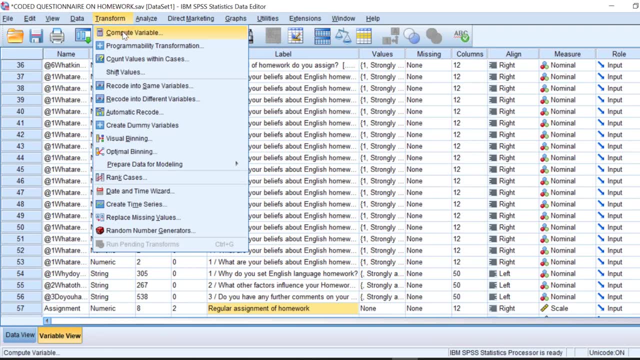 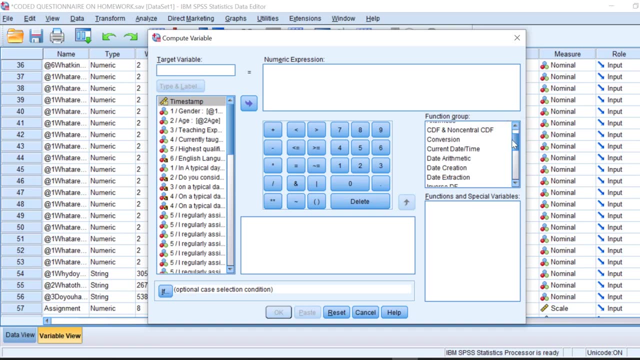 items into one variable or different variables. so I'm going to show you the first way we can go to transform and then compute variable, and I'm going to find all the functions that can be identified from this box. here we have statistical scoring, strength, time search, etc. I'm going to choose. 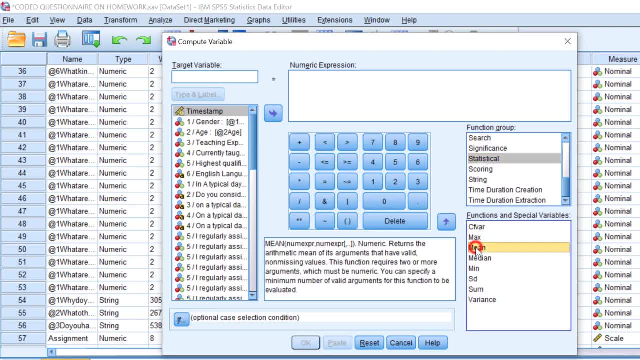 statistical, and then I can choose either the mean- I move it, or I can choose the median and I move it here. so anyways, I'm just going to show you the mean function. once I choose the mean function, I can just copy these items and paste them here, or rather, I can like not. 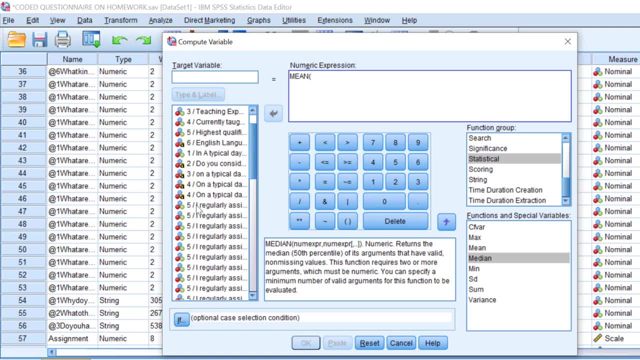 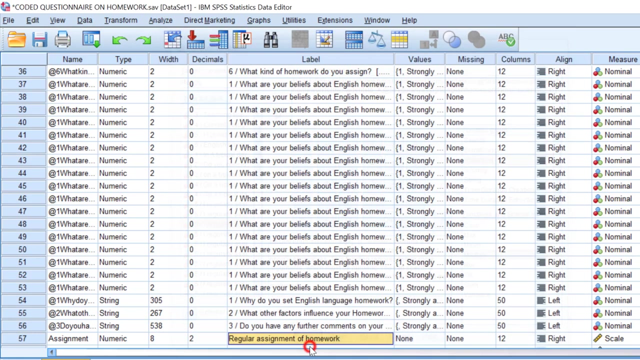 copy, just drag them and drop them here. otherwise I can double click like this, but I need to keep adding commas okay, till I finish all the items. so once I finish them I need to close the parenthesis and click OK. but before that I can give it a name like regular etc. then click OK. so once I click OK, the 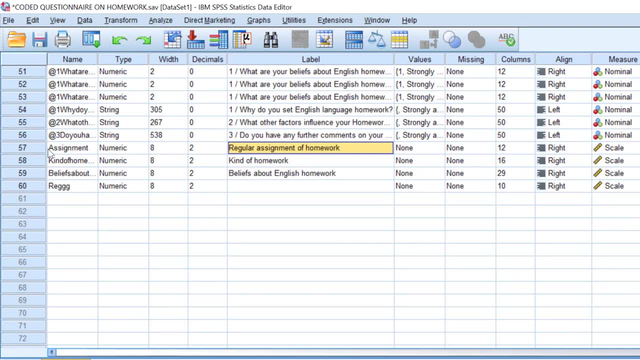 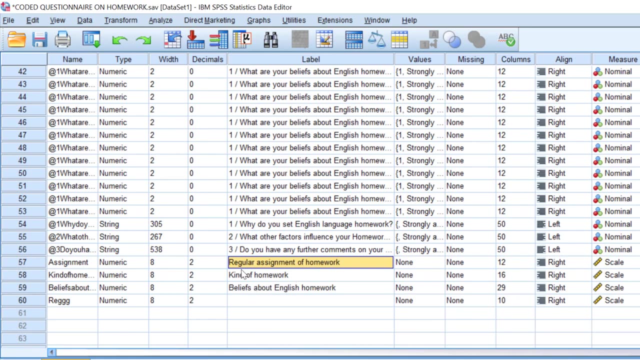 variable will be created at the end of the data or the variable view and even the data view here. so anyways, we can, once I group all of them based on the mean, I can compute their means score so that I can group them, for instance, so I can go. 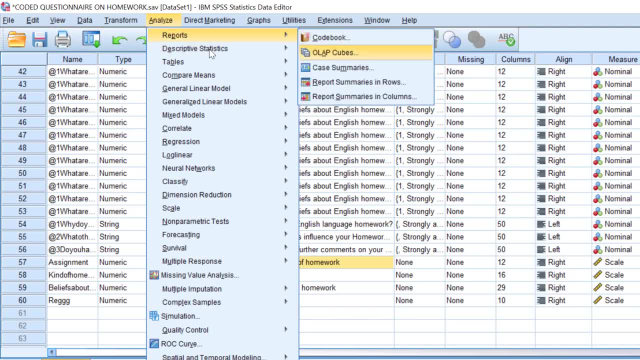 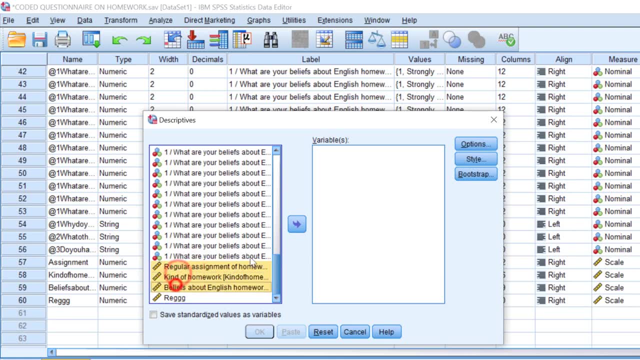 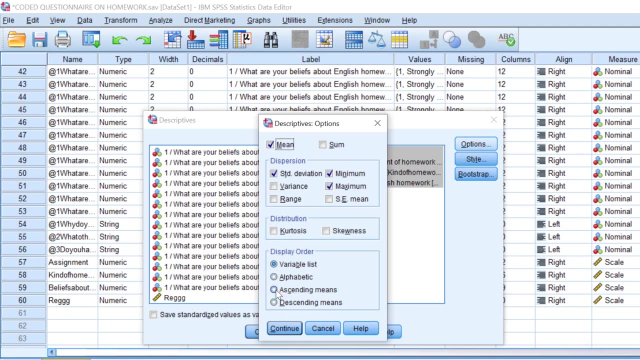 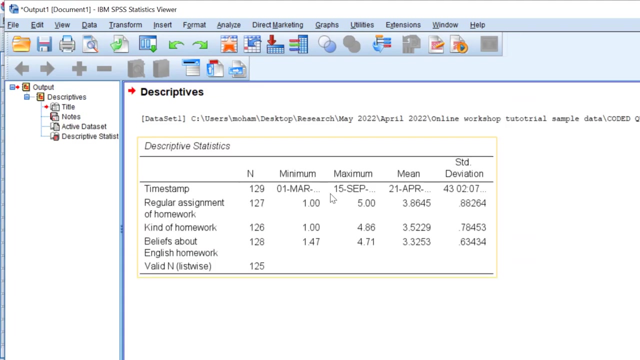 here to analyze descriptive stats and descriptives and I need to move the newly created variables like this. but in options I need to choose ascending means, so this grouping here can be based on ascending or descending means. let's choose, for instance, descending means, click continue, click OK and you can find the, the scales, grouped based on the descending means. 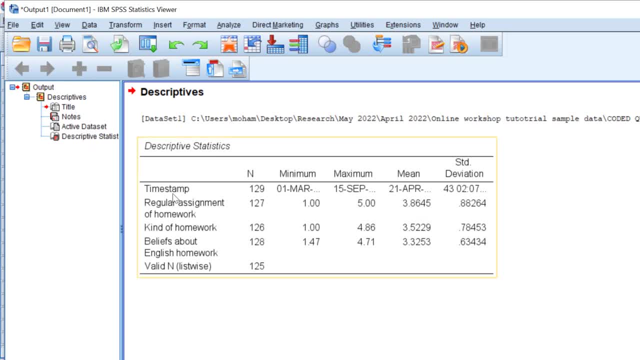 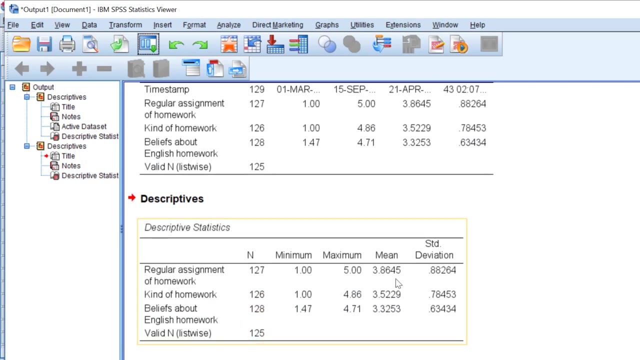 for instance like from the highest to the lowest. so I just miss move this, let's say timestamp. I can go back descriptives, remove it, click OK this way. so this is the first way I can group the lacquered scale items. the second way is: 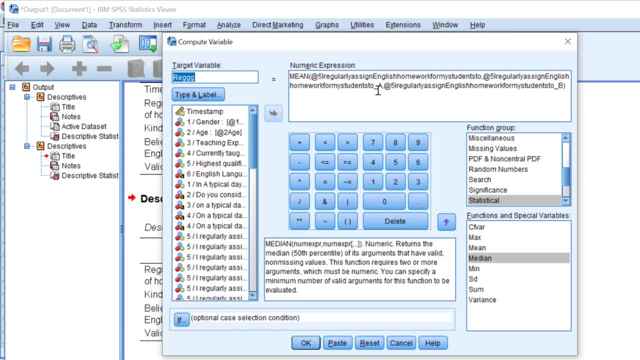 through transform compute variables. but I'm going to choose the median, not the mean. if I can't find the mean here or the median, I can just type it. so I can type it using: I can type it using uppercase click open parenthesis and I move the items till I finish, one by one. 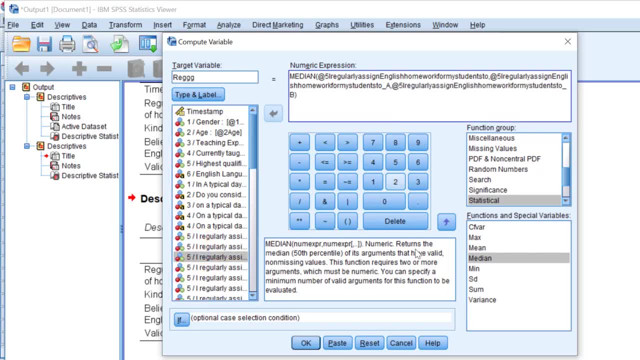 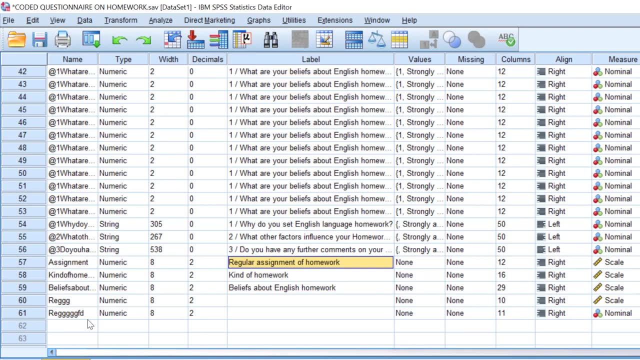 till I finish and then close the parenthesis and then click OK again. a new variable will be created at the end, but this is the median. so the mean score is used when we use parametric statistics like t-test, ANOVA and COVA. is used when we use parametric statistics like t-tests, ANOVA and COVA. 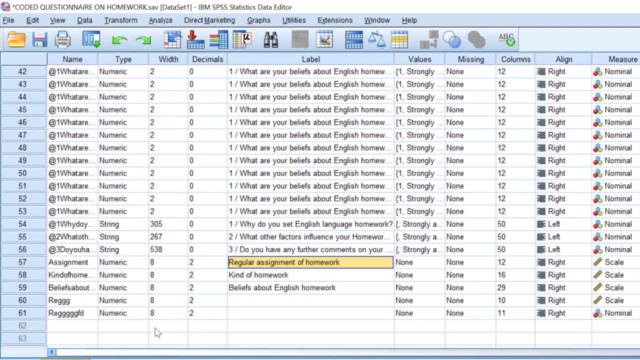 linear regression etc. but the median is used mostly for non parametric tests, like the man with nu test, cross-co-horn, wallis edge tests, ordinal and logistic regression etc. there are like two ways of how you can group the lacquered scale items into categories so that you can run other tests subsequently. you can 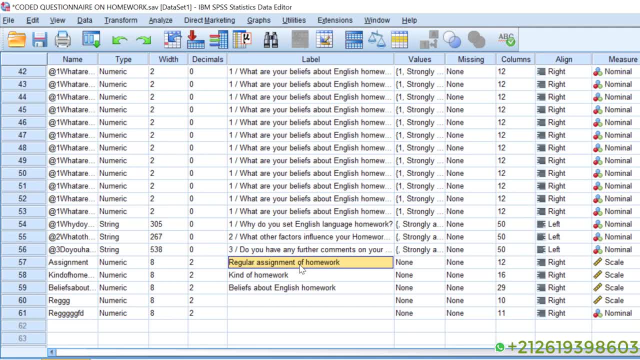 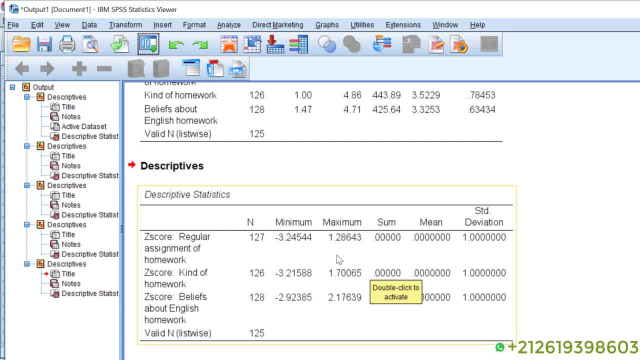 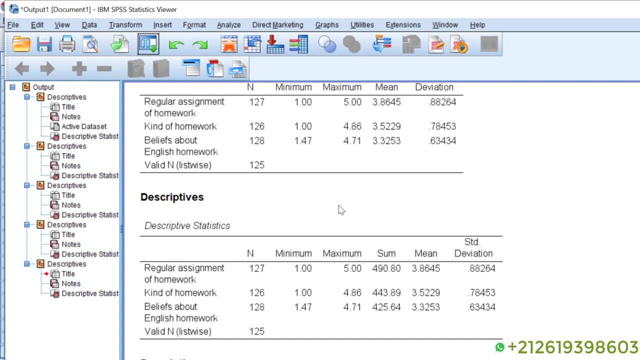 either run descriptive stats by grouping or by, let's say, classifying the items based or the scales based on their mean score or based on their median score. so these are like different ways of how we can in fact group lacquered scale items. you can choose the way that suits you the best and, if you have,